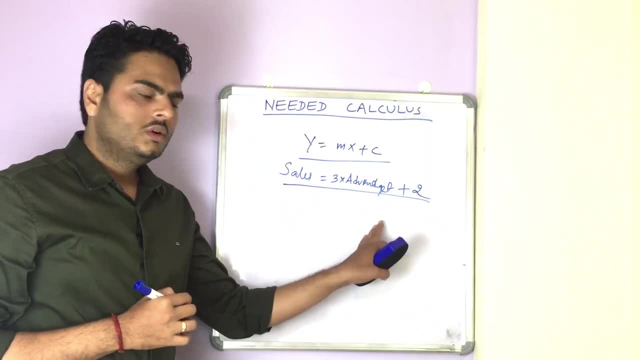 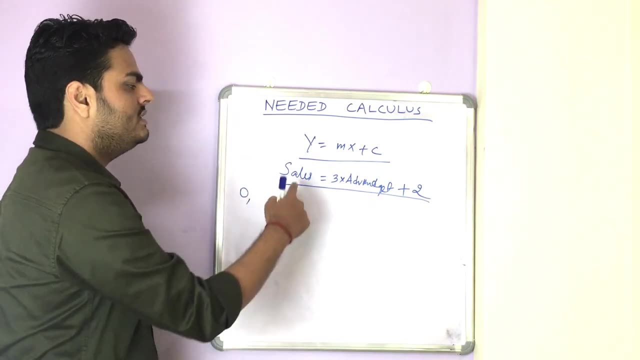 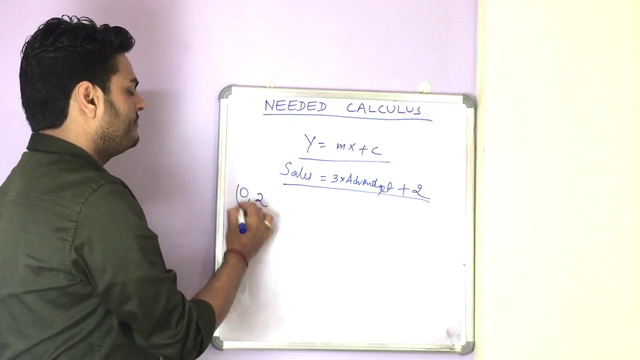 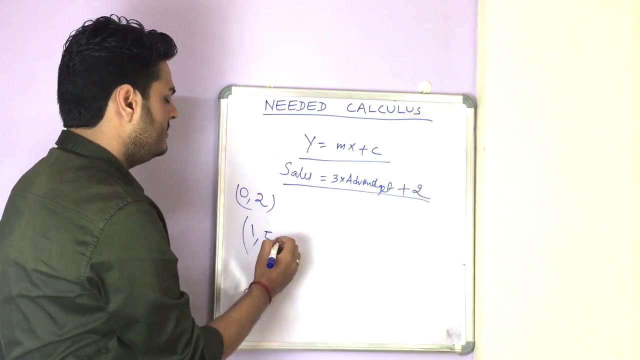 this relation. What is the meaning of this straight line is: whenever advertisement budget is 0, then sales becomes 3 into 0 plus 2.. So how much sales becomes 0 plus 2? 2. Whenever advertisement budget is 1, then sales becomes 3 plus 2, 5.. So 5.. When budget is 2, then sales becomes 3 into 2, 6 plus 2, 8.. 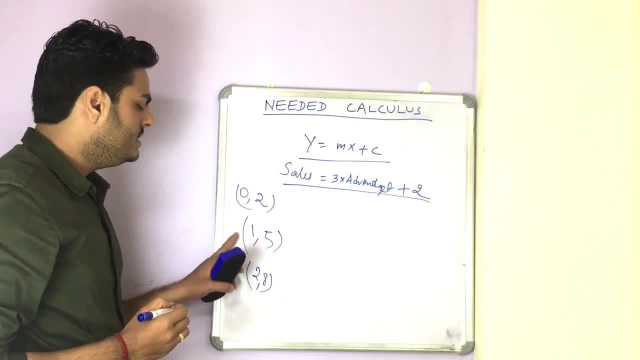 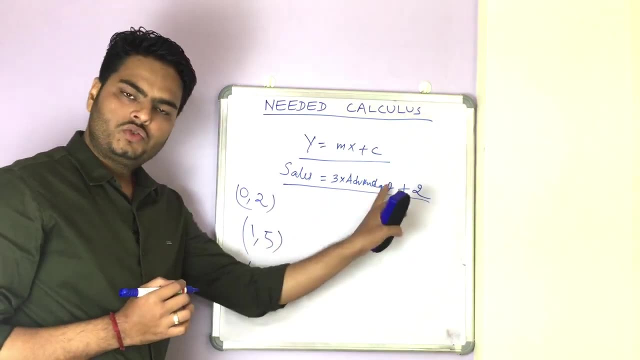 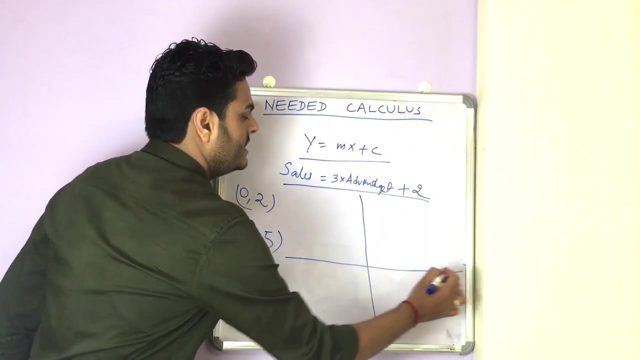 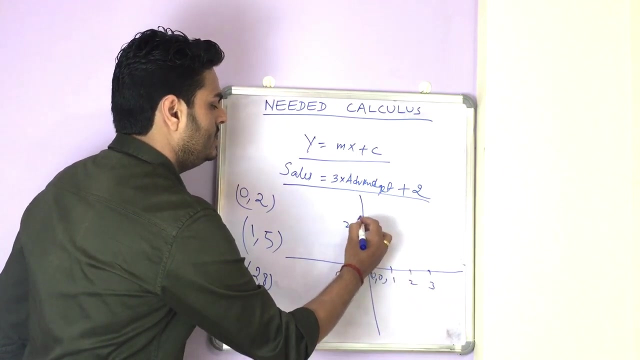 2 and 8.. So these three are the points of straight line represented by this equation. Now let's try drawing the straight line on xy plane. So just imagine: this is the xy plane and this is the origin. This is positive: x 1,, 2,, 3.. This is positive: y 1,, 2, 3, and these are 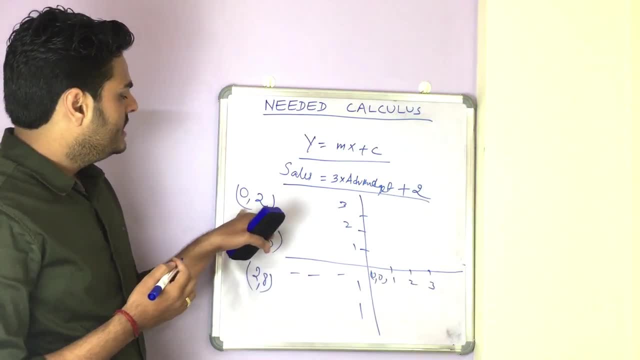 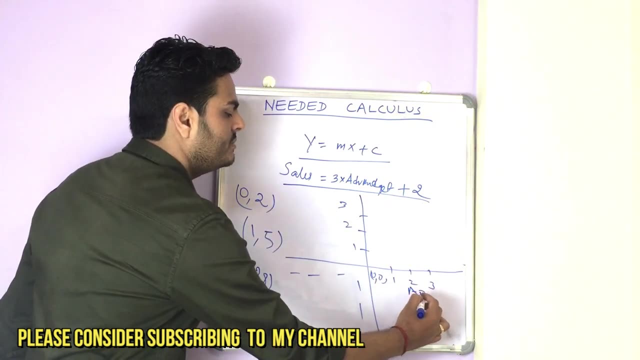 negative x and negative y. Now if we have to draw 0, 2, then where it will come. When x 0, then y is 2.. So in this case x is advertisement budget and y is sales. So when x is 0, then 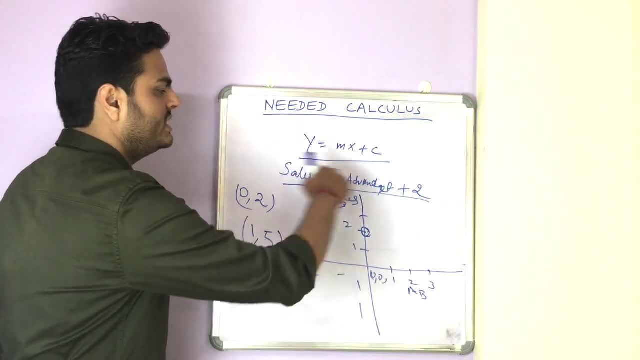 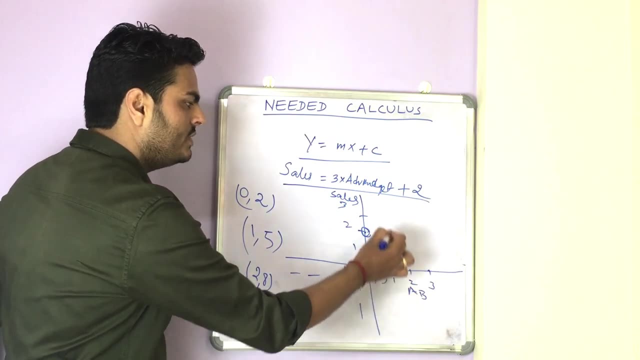 y is 2 means- this is one point on this line, this particular line- When x is 1, then y is 5.. So this is your x. When x is 1, then y becomes 5.. So I have drawn up to 3 here only, Let's. 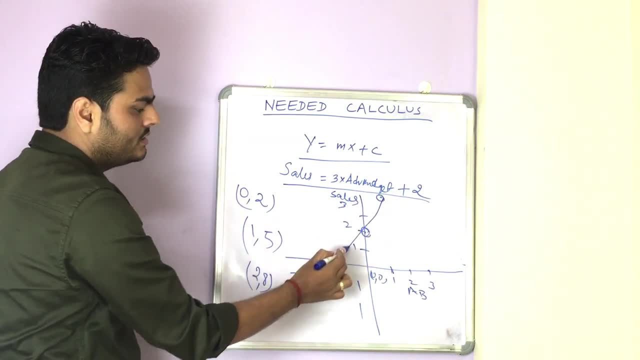 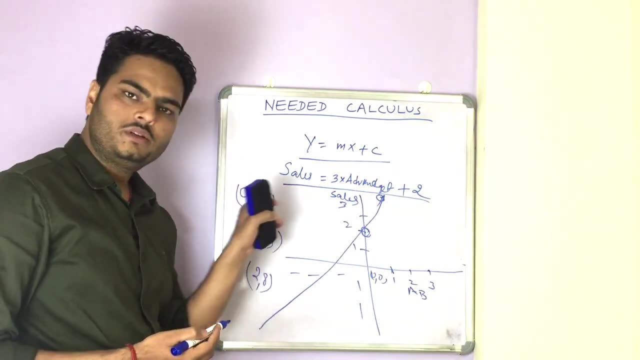 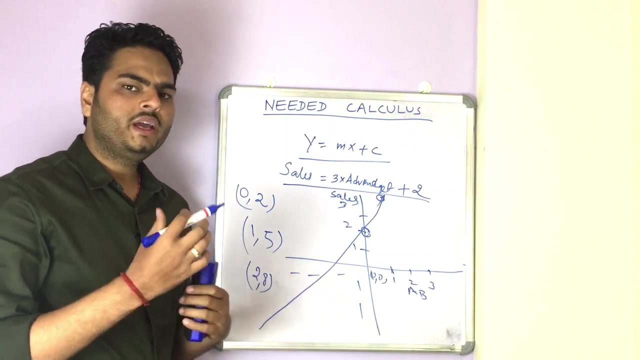 say, this is 5.. So your line will look something like this: Now, this line is illustrative, So this line here is illustrative. So you can see that this line is as another line. It is a line which is representing this imaginary business. 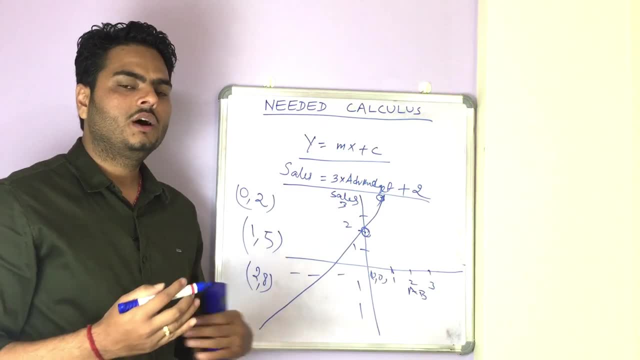 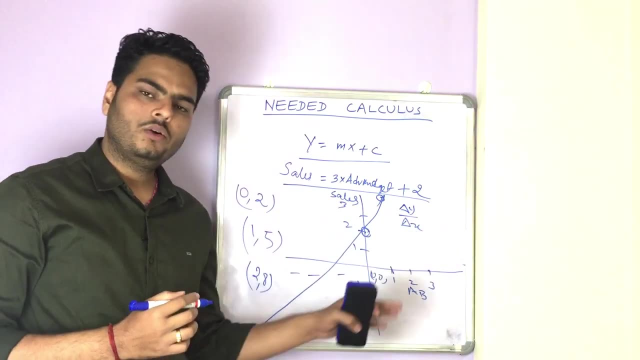 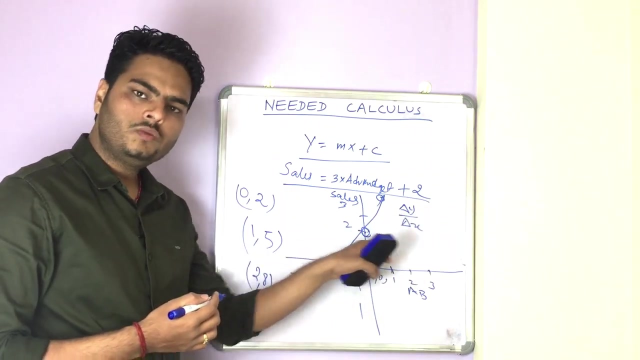 that we are talking about Now. one important thing to note here is how y is changing with x or with the shift in x, How y is shifting. That is called delta y by delta x. So what is the rate of change of y with rate of change in x? 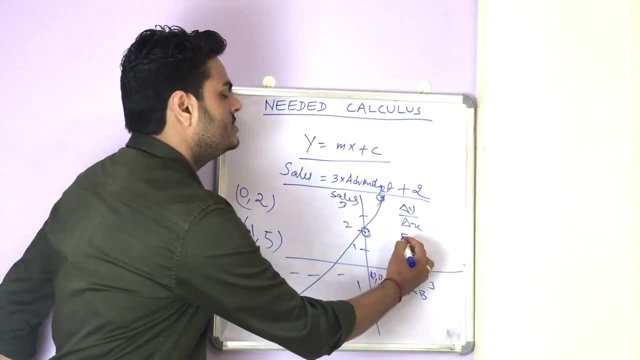 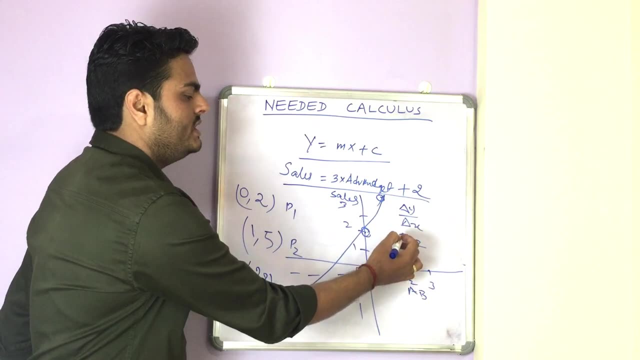 that is changing Two values of y. let us take 5 minus 2. delta y change in y. I am considering these two points, p1 and p2.. So delta y is 5 minus 2 and delta x is 1 minus 0. So if you take this, 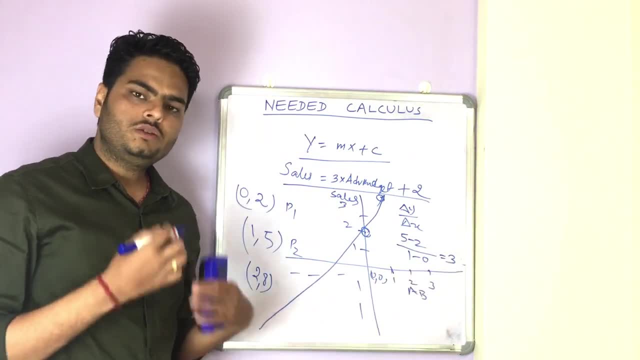 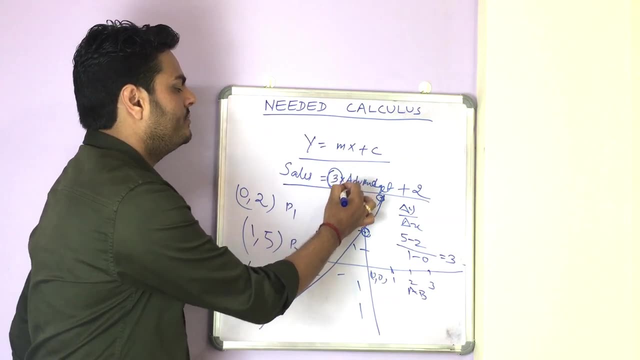 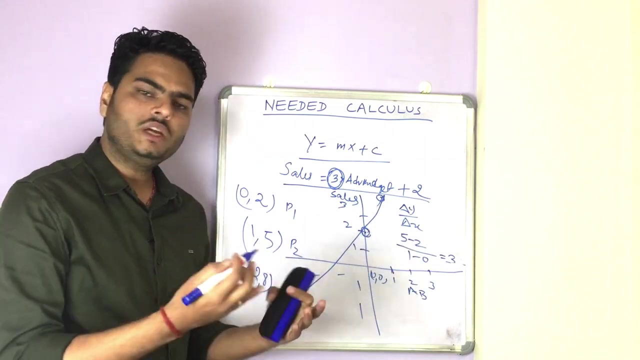 and if you evaluate this will be 3, which means 3 is the slope of this line. Now, if you go to this equation, here I have manually placed 3.. So this 3 and this 3 are same, which means that for every unit shift in x, y is shifting by 3 units. Now the interesting thing is, in this straight line, 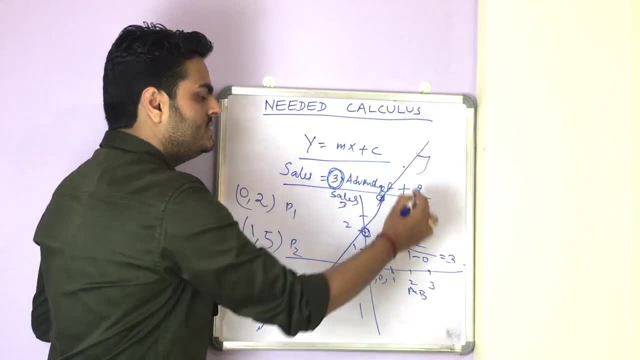 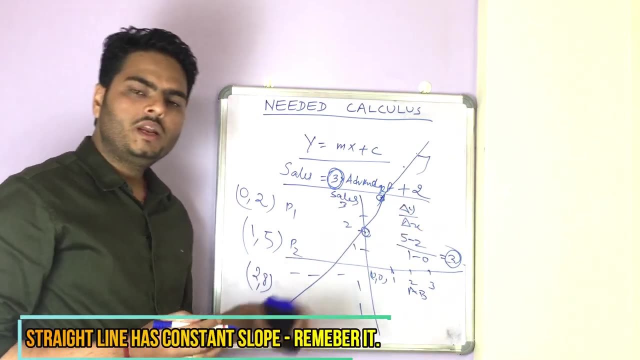 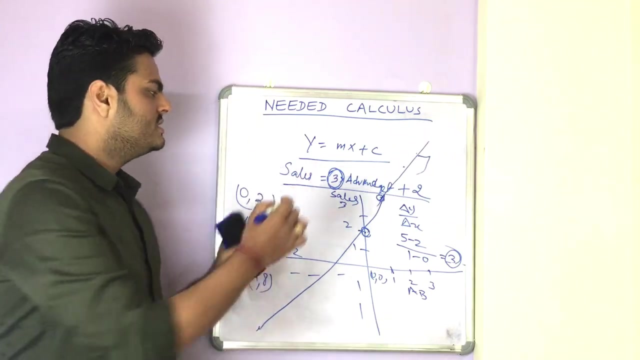 anywhere you go, any two points you take, this shift will be constant. So for every unit shift in x, y will shift by 3 units. This is valid till we are talking about a straight line. But how many businesses will have this kind of scenario? Business scenarios are very complex. 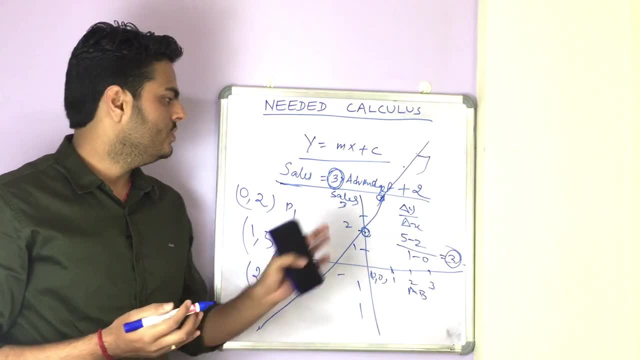 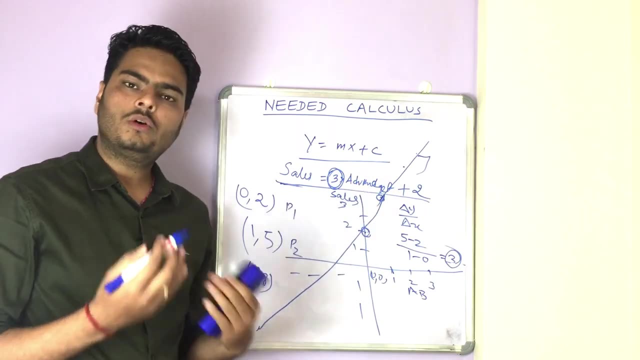 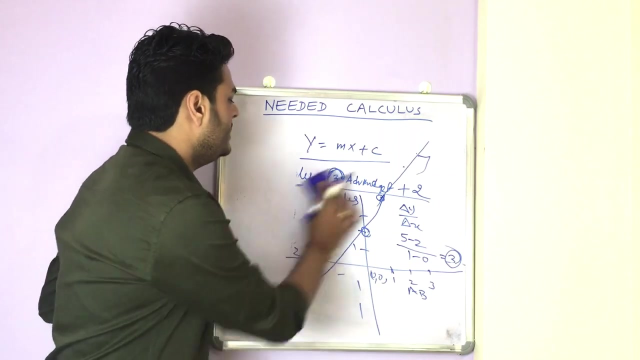 than this. So none of the business will, you know, follow a straight line equation like this. Hence, in the world of data science and machine learning, we have more complex equations, And that is where calculus helps us. I will tell you how. Now let us say, in place of this: 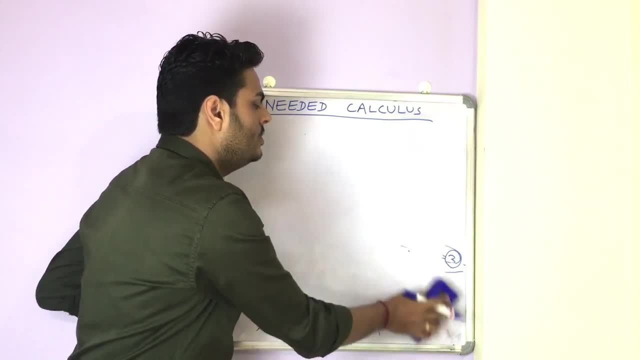 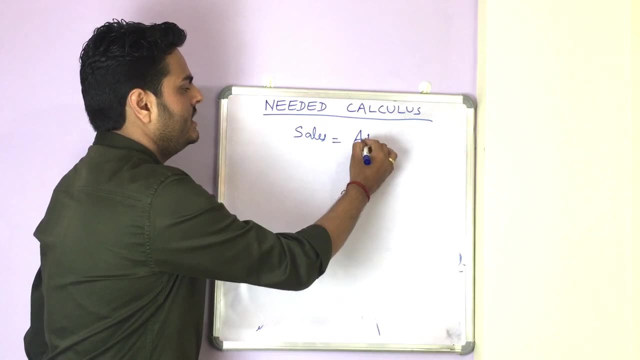 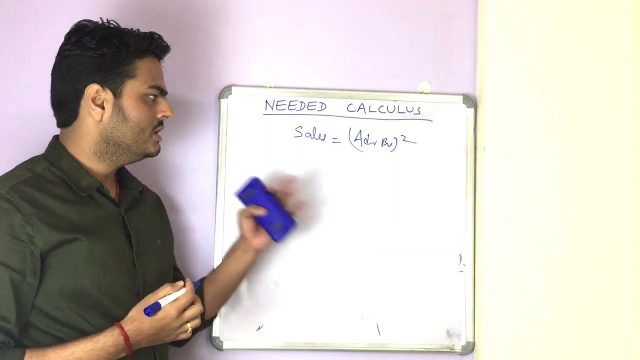 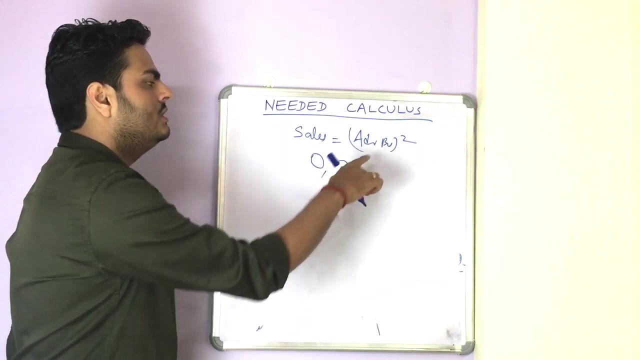 straight line equation what we are talking about. We have a relationship between sales and advertisement, as sales is equal to advertisement budget square. Possible it can happen, just an imaginary situation. So what will happen here? when sales is 0, when advertisement budget is 0, sales will be 0.. 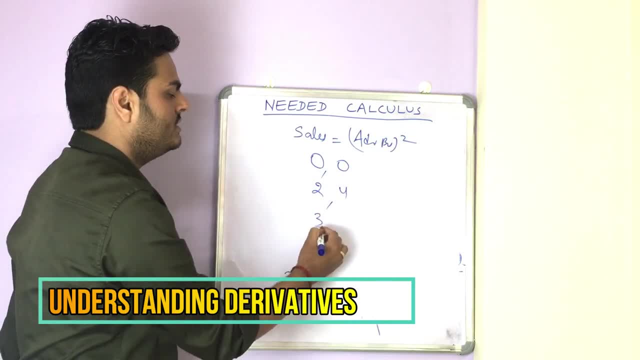 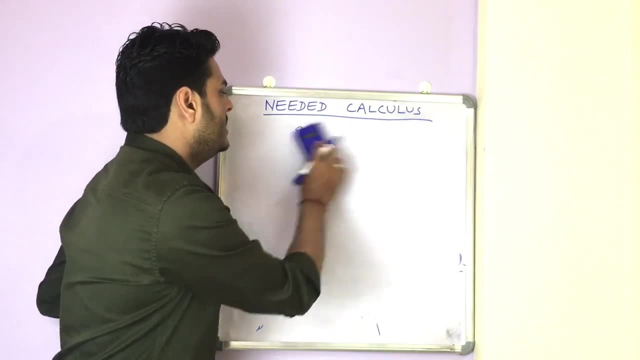 When budget is 2, sales will be 4.. When budget is 3, sales will be 9.. This is a square function. Now let us try understanding how this square function will look like in x- y plane. So if this is your x- y plane, 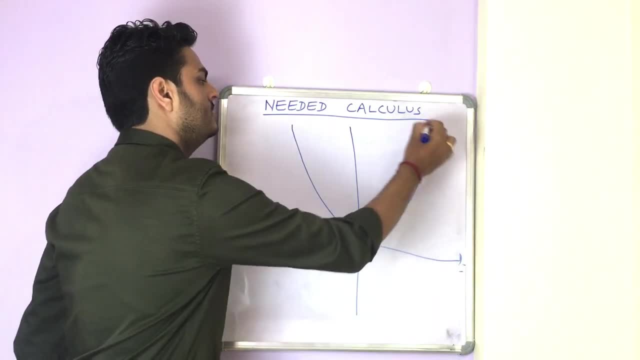 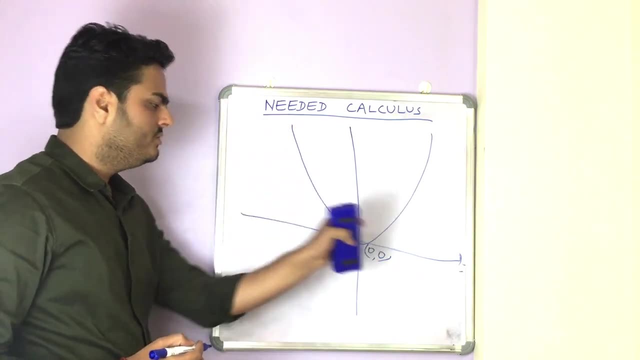 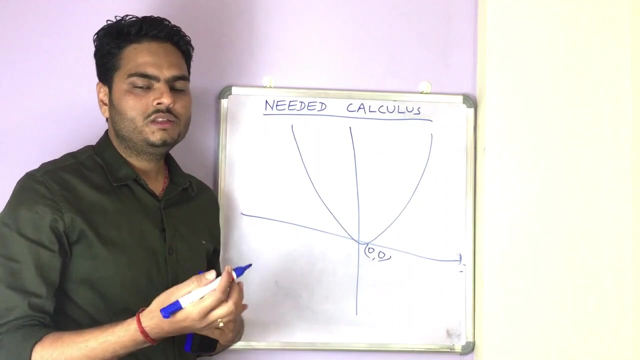 then the square function typically looks like this. So this is your origin: 0, 0. even for negative x's, your y is positive and for positive x's, your y is positive. But it's very important to know how y is changing with x at different points. Now 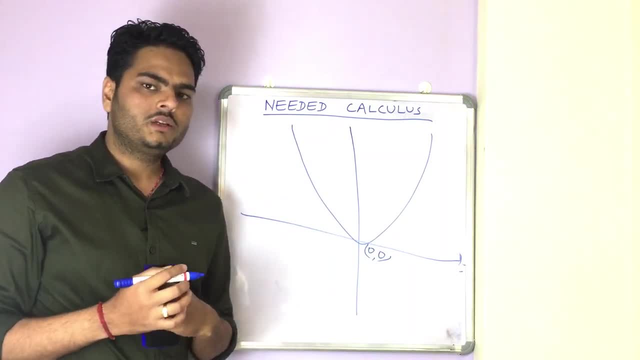 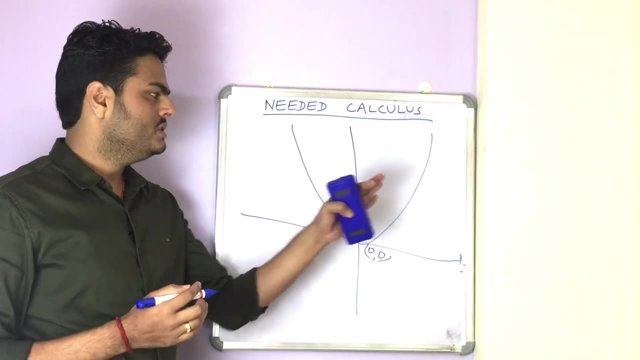 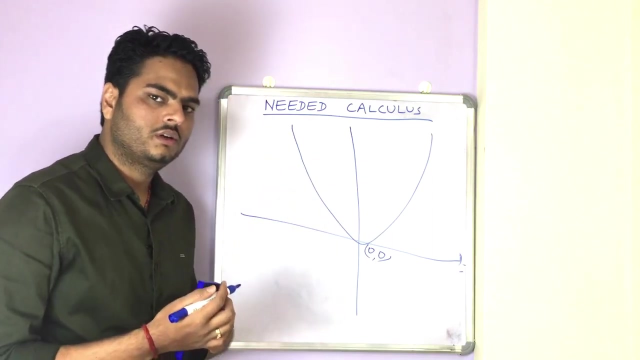 if you remember, in the equation of straight line I told that all the points has similar slope or similar change in y with respect to change in x. Any point you take, the slope remains constant. But in this parabola the slope is not constant. Here the slope will be different. 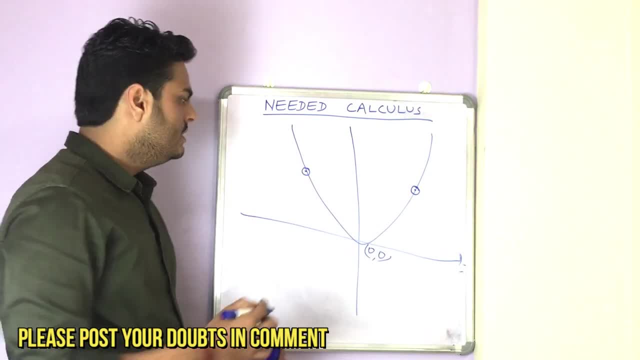 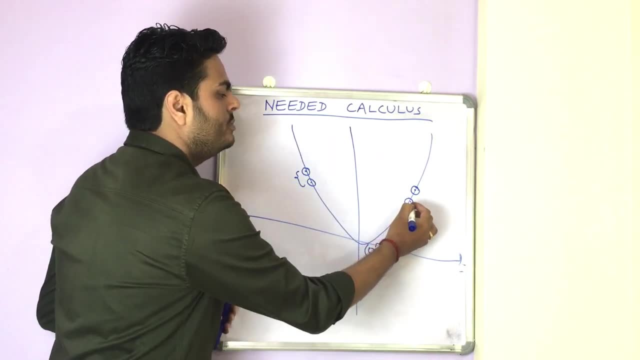 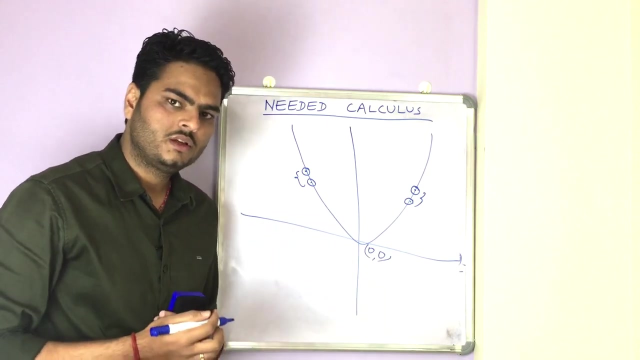 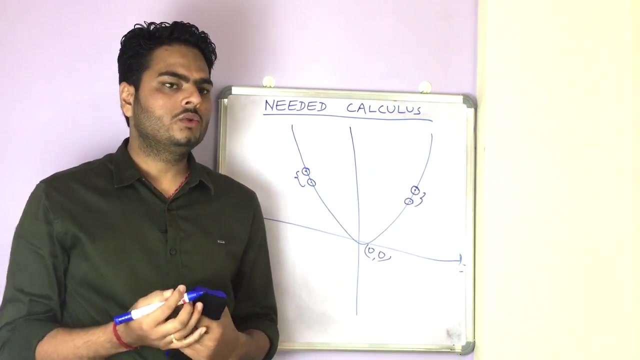 and here the slope will be different. So if you calculate slope between these two points, it might be different or it is different. Then slope between these two points. This is a complex situation where calculus helps us and it is very important to know at what point what is the slope, so that we get to know. 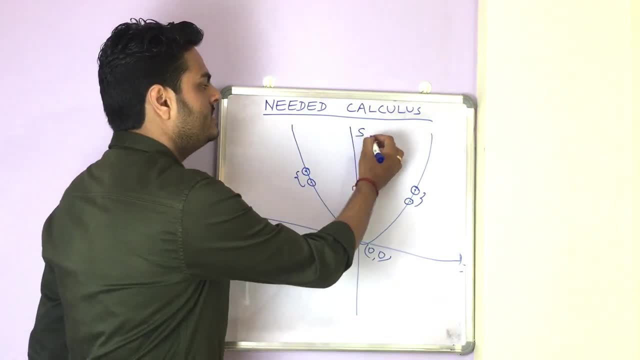 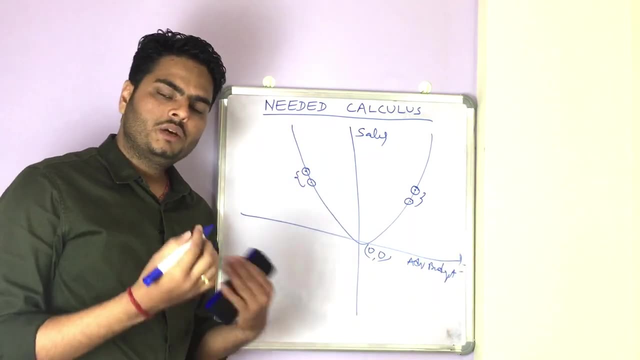 in which direction y is moving. Now imagine this is your sales and this is your advertisement budget. So for a business, it becomes very important to know up to what limit is your sales. So for a business, it becomes very important to know up to what limit. 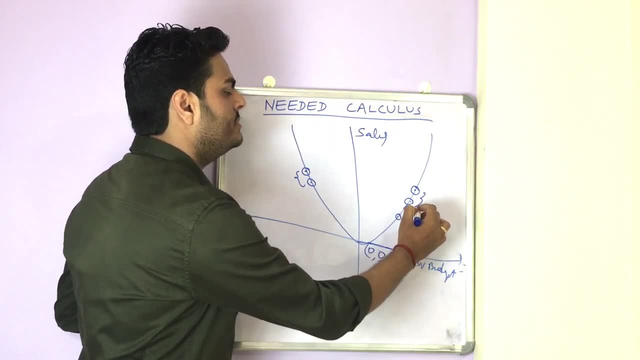 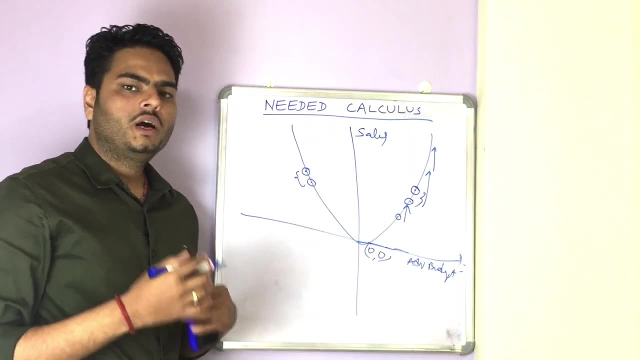 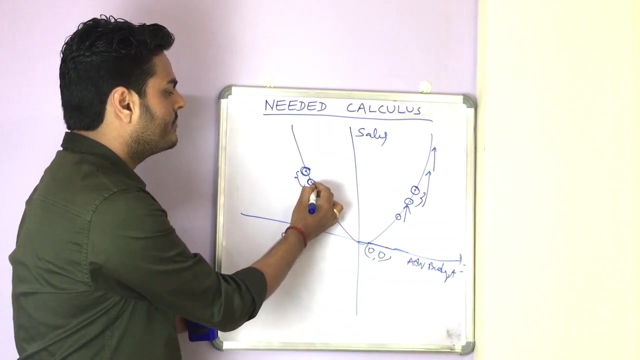 I should spend so that my sales keep going up, and it goes up by a significant amount. Let's see with example how calculus solves this problem. So if I consider these two points here, let's say this point is x and this shift is very minimal. 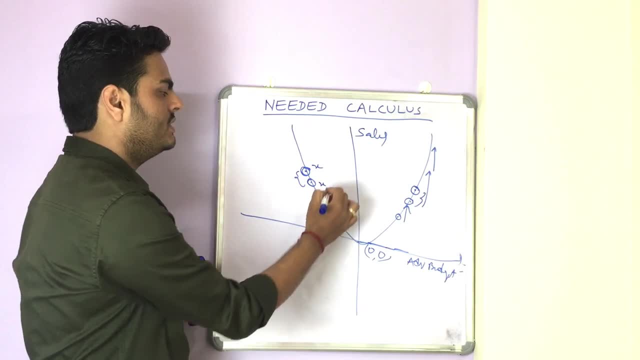 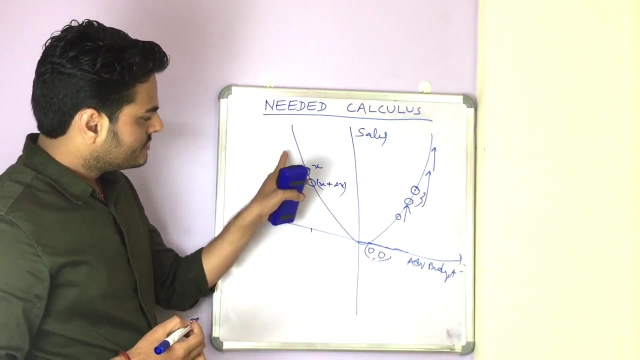 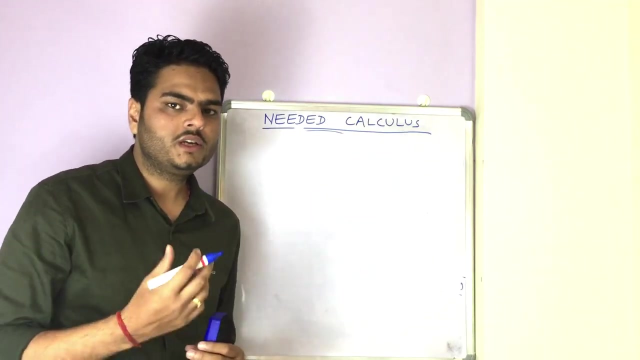 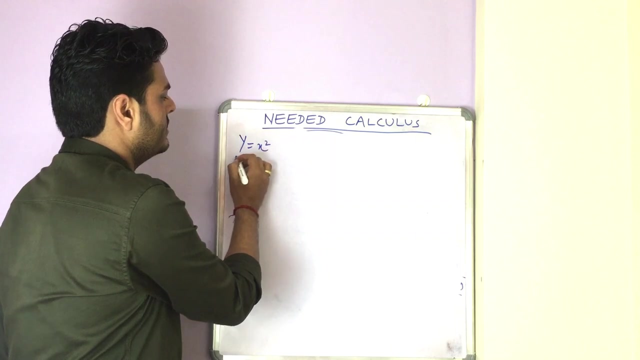 Let's say on x-axis- on x-axis I am talking about- this is x plus delta x, where delta is a small number. now, when x shifts from x to delta x, then how y is changing. let's try calculating this shift in y with respect to shift in x. so my original equation is: y is equal to x squared and I: 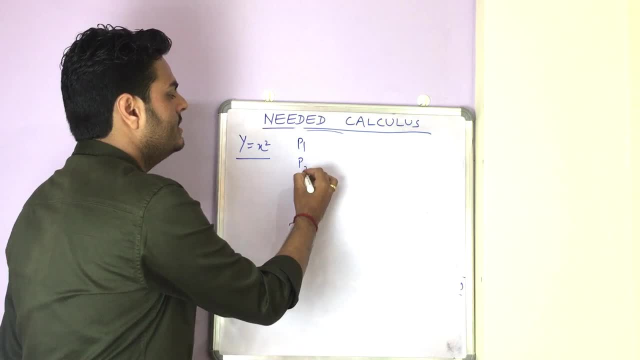 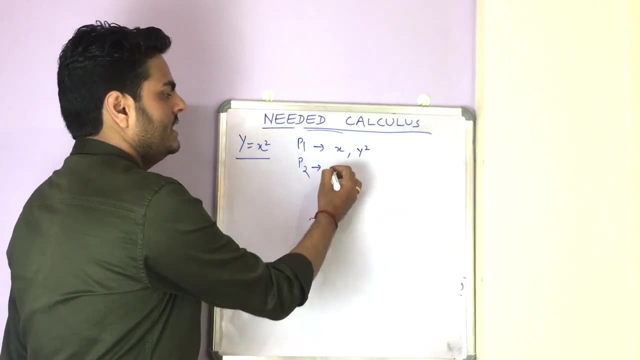 am considering two points, p1 and p2, so in P1 the value is x and the value is y square, whereas in P2 I am just shifting x by little bit so that I can calculate the slope. I am saying x plus delta x. 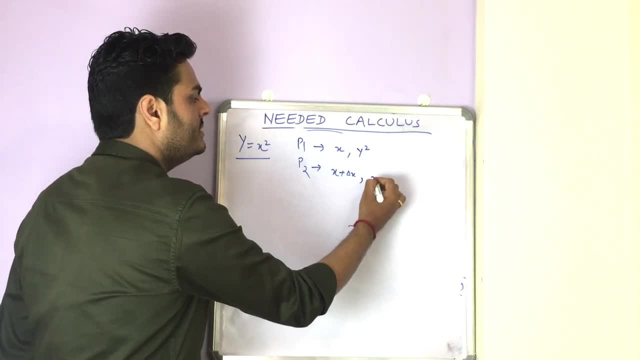 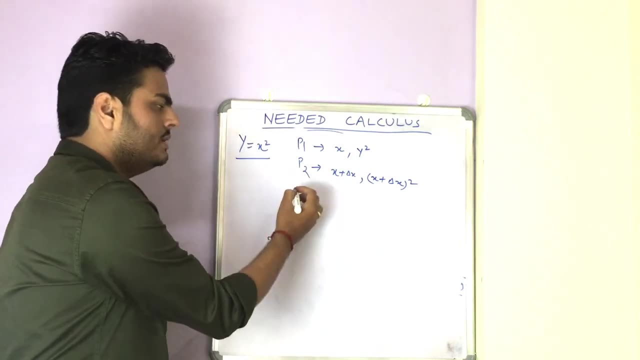 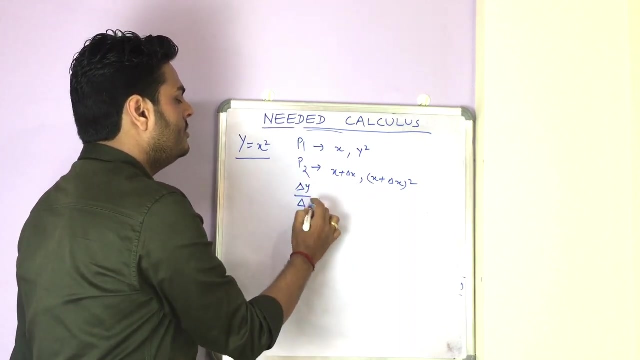 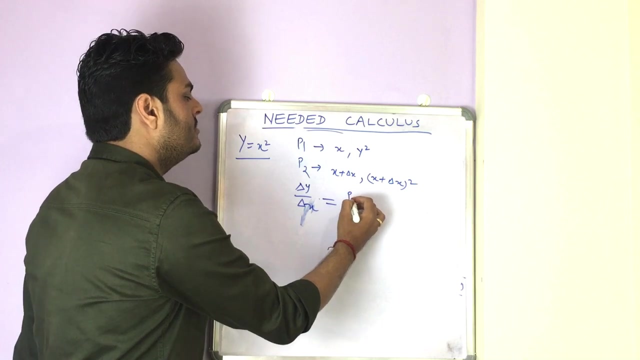 well, delta x is a small number and hence y will become x plus delta x, whole square. right Now, if we have to calculate delta y by delta x, which means I want to calculate how my y is changing with changing x, So I should substitute the values here. I will say p2 minus p1 y values. 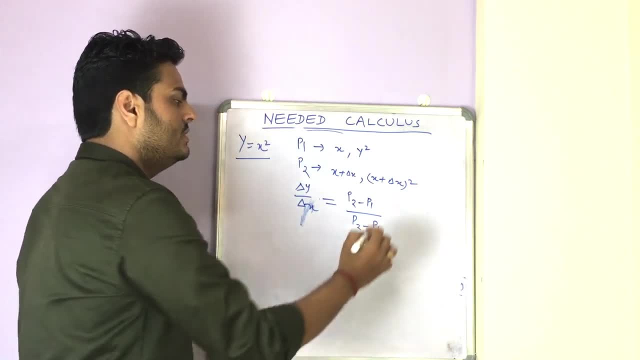 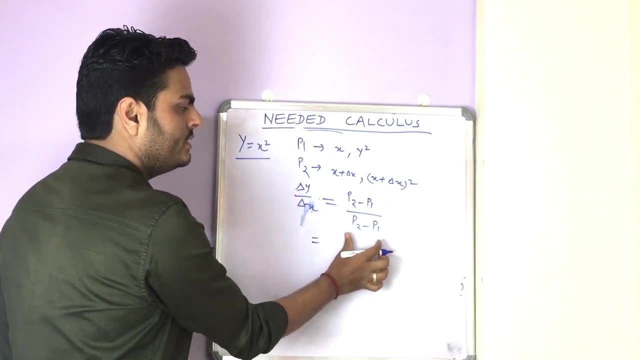 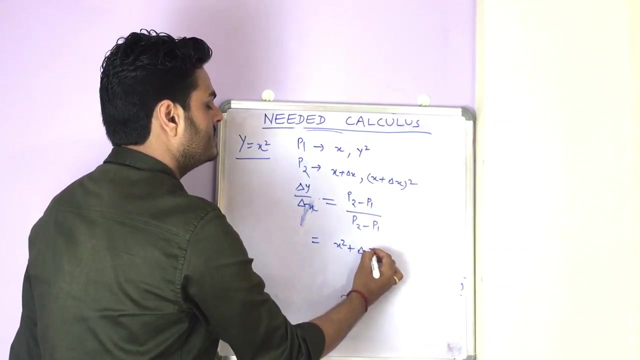 by p2 minus p1 x values. So this will become: we have to replace the values x plus delta x whole square because numerator y values. So x plus delta x whole square will be x square plus delta x square plus 2x delta x. 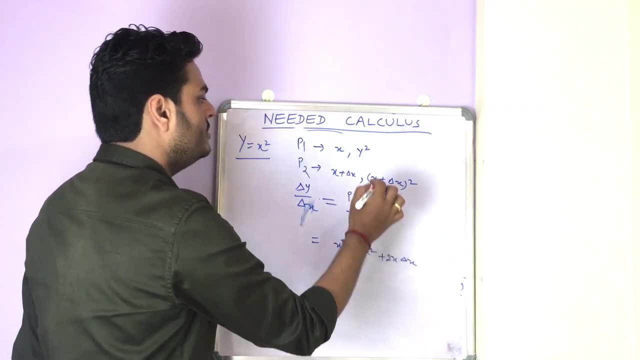 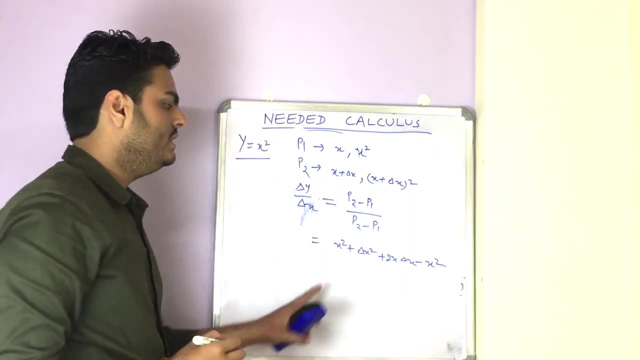 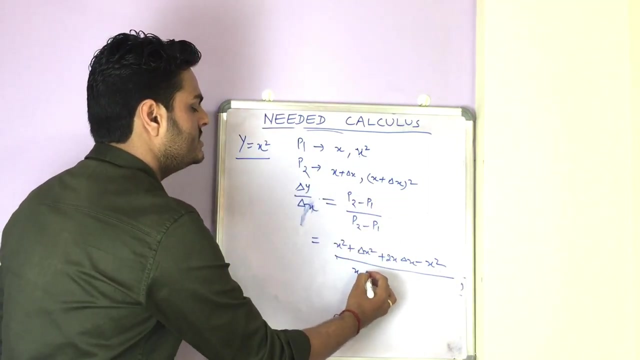 Right, and what was the previous value? So this will be basically x square. So what will be the previous value? It will be minus x square right, and then in the denominator we have to write the x values. So what are the x values? x values are x plus delta x minus x. So x plus delta x from. 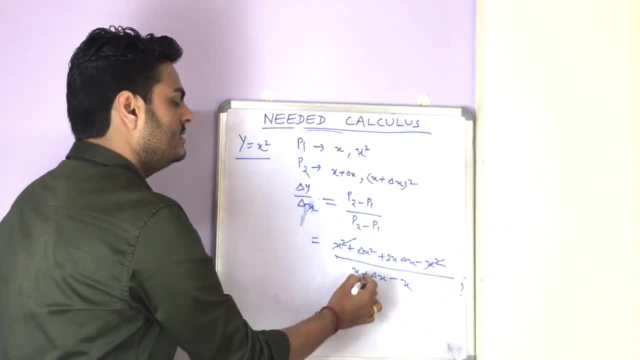 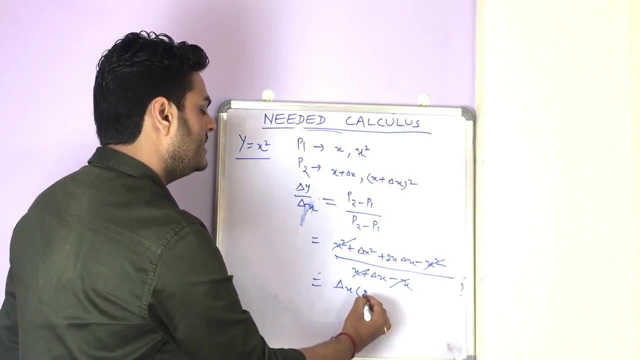 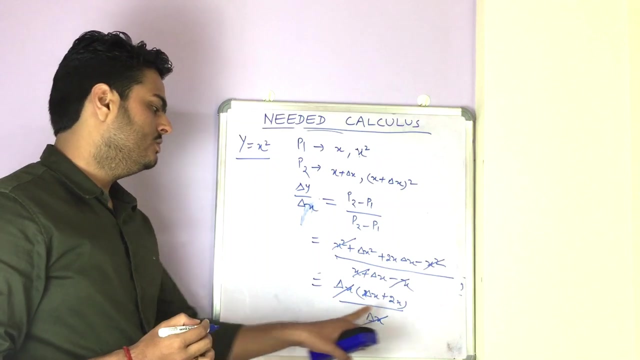 here, x. from here, These two things get cancelled. These two things get cancelled. if you take one delta x out from here, So x plus delta x from here, x from here, So x plus delta x from here, x. from here, it will become delta x plus 2x divided by delta x, Delta x, delta x gets cancelled. So what? 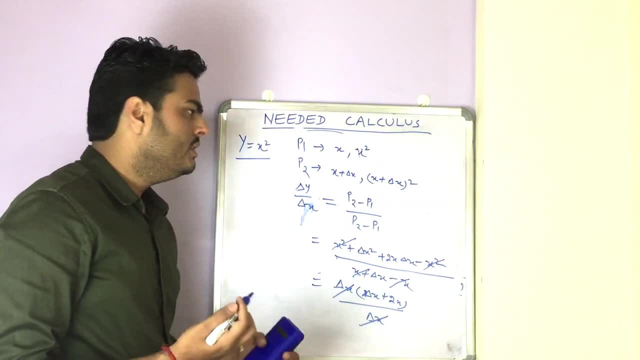 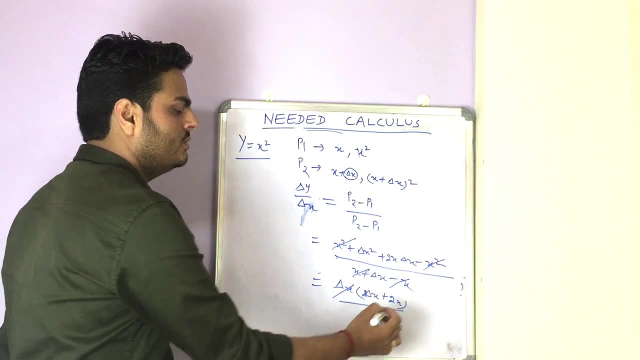 we are left with is delta x plus 2x. Now, as I told in the beginning, this delta x is a very small number. So what happens? if this delta x becomes 0, then this becomes 2x, So this 2x is known as. 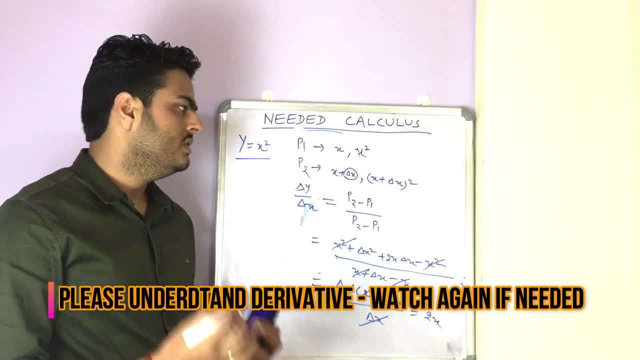 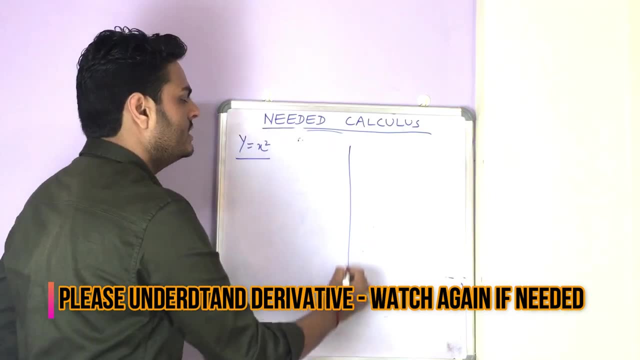 derivative of that curve. So this 2x is known as derivative of that curve. So this 2x is known as any given point. Now, this is the curve we are talking about. guys, If you want, you can rewind and see once. This is the curve we are talking about. What we have just derived is the slope. 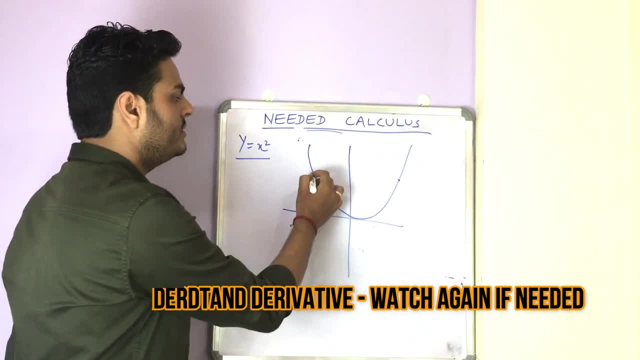 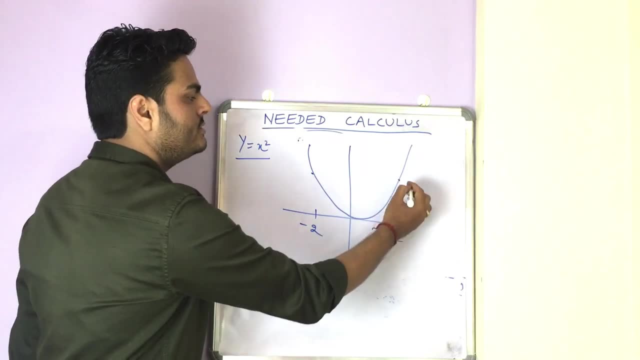 of this curve at any given point. Now let me take two points here. okay, So this is, let's say, positive 2.. This is, let's say, negative minus 2 on x axis. So what will be the slope here? 2 into 2. 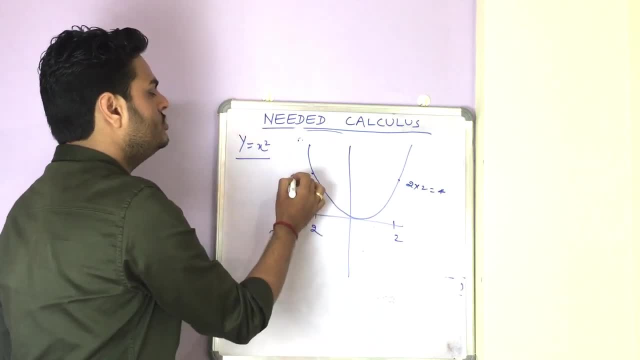 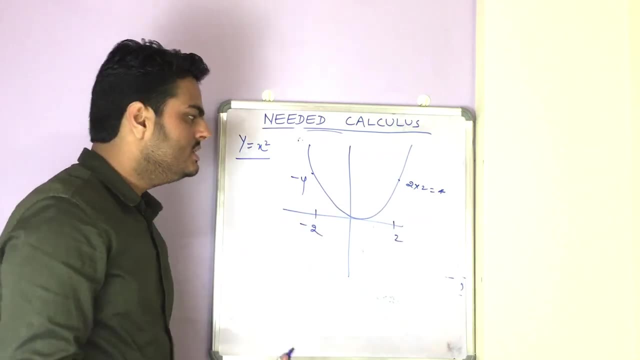 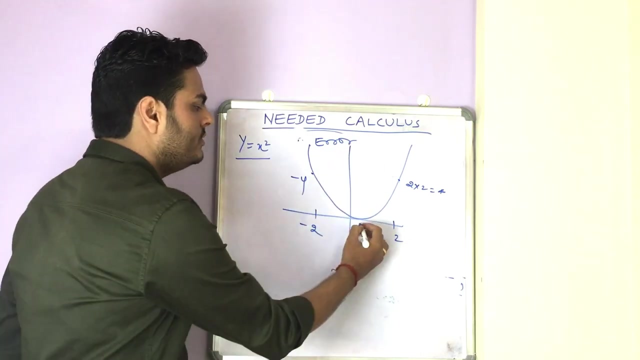 is equal to 4.. And what will be the slope here? 2 into minus 2, which is minus 4.. This is very, very important in the world of machine learning and data science. The reason is, let's say, this is error of your machine learning model. okay, And this is one of your variable in. 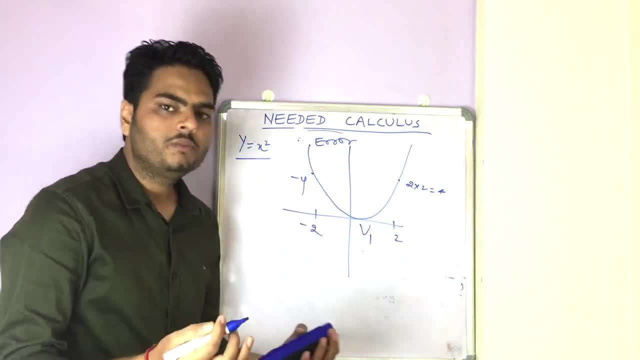 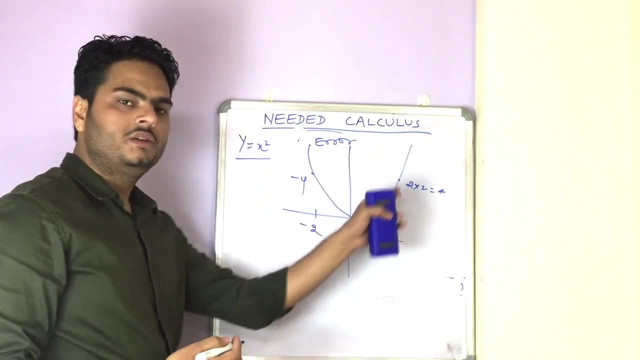 the data. Let's call it variable 1.. So we want to optimize what should be the optimal value of v1, so that the errors are minimized. So where is the error minimized? Now, here we can see and say: this is the place where error is minimized. But when equation becomes complex, 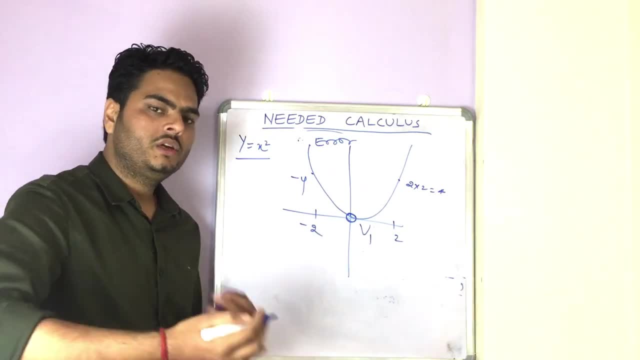 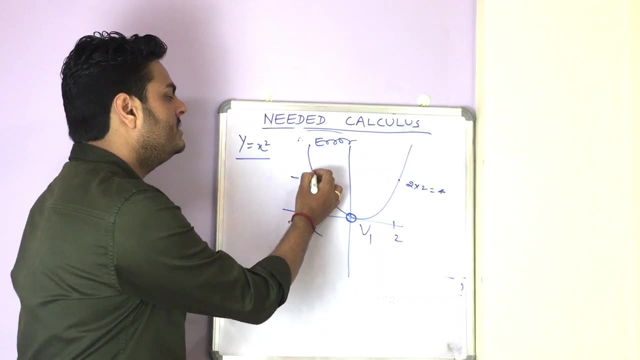 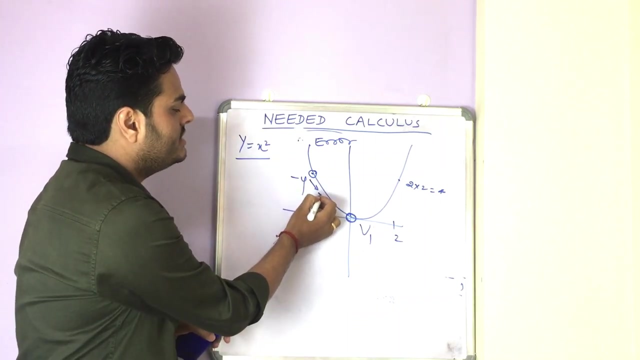 then, point by point, we have to go and iterate till we reach the minimum value. But how do we know in which direction we have to move? For example, if I start from here and it's a negative slope, then we know that error is decreasing in this direction with increase in x, which means this: 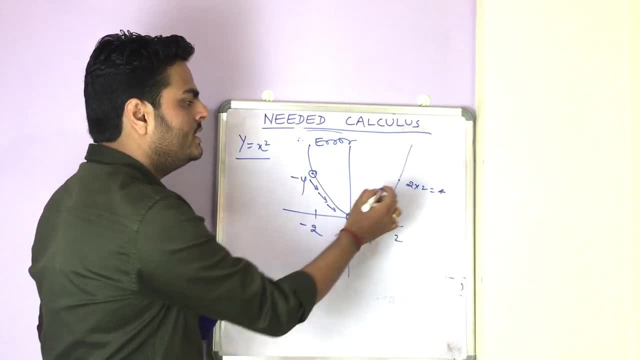 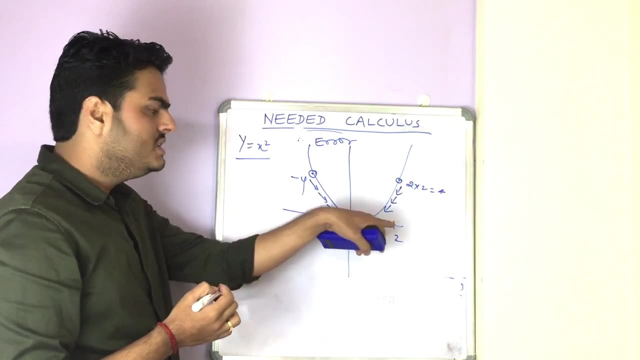 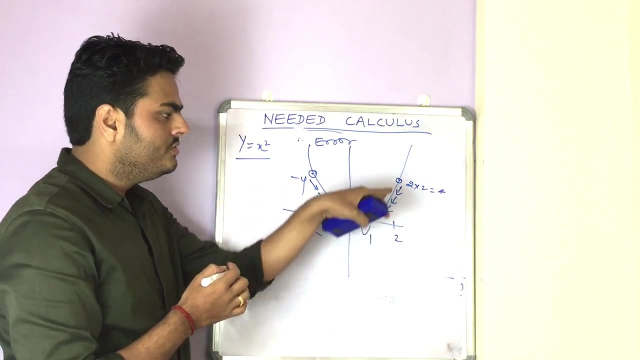 is the direction we have to move. okay, On the other hand, from here, if we move to this direction, then we know error is decreasing with decrease in x And hence, in this case, if we increase the x, error is decreasing. In this case, if we decrease the x, error is decreasing And hence there is a. 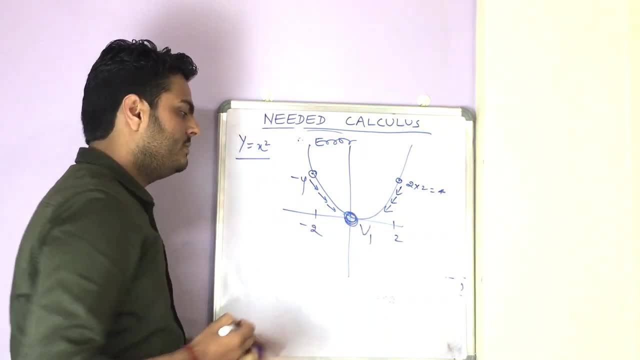 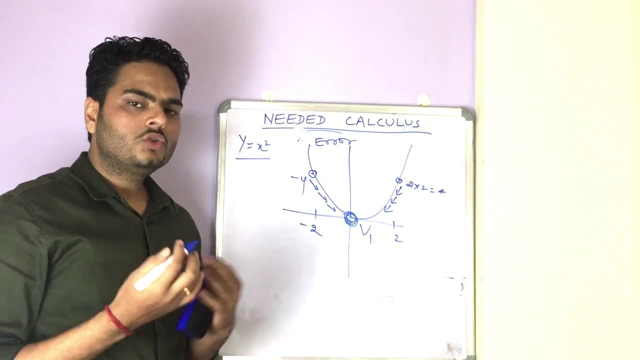 possibility that we might reach to this optimal point, And this is what we intend to do in machine learning. So this is a very important concept if you talk about so many optimization problems, so many error optimization problem And this 2x that we just 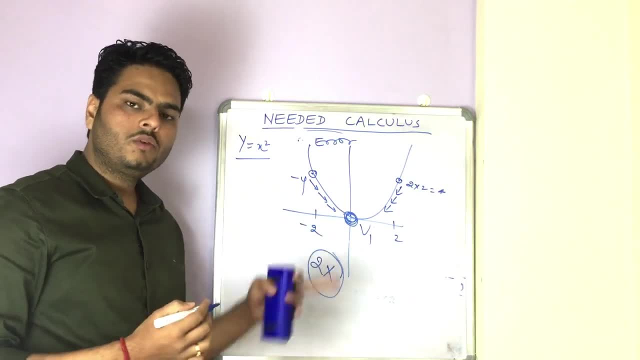 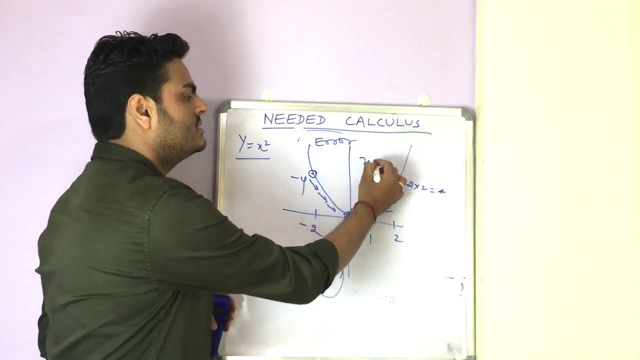 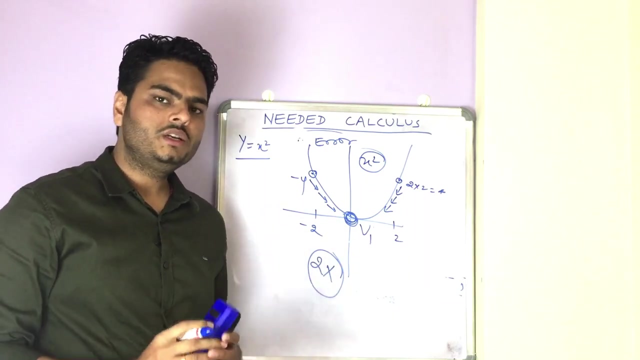 derived is known as derivative of that curve at any given point. This is also known as differentiation of this equation. In this case, equation is x square. okay, So this is about one part of calculus known as differentiation. Now let's talk integration. okay, So if I give you a square, 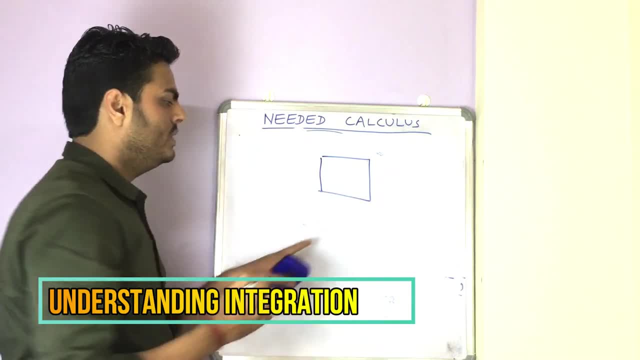 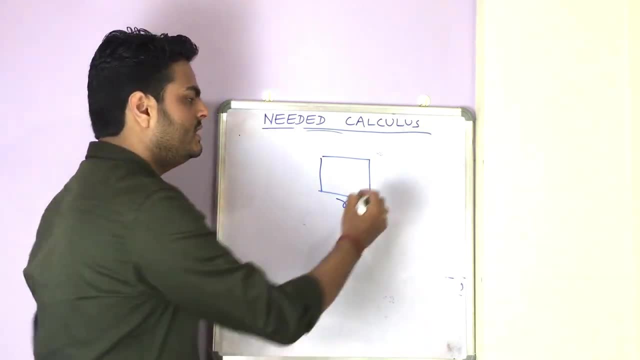 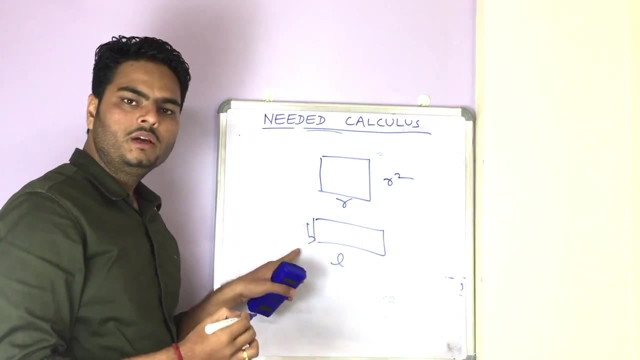 and I ask you what is the area of the square. I tell you r is the length of the one side. So you will tell me r square. If I give you a rectangle, you will tell me what is the length and breadth. I say you l and b and you can tell me l into b is the area of this rectangle. 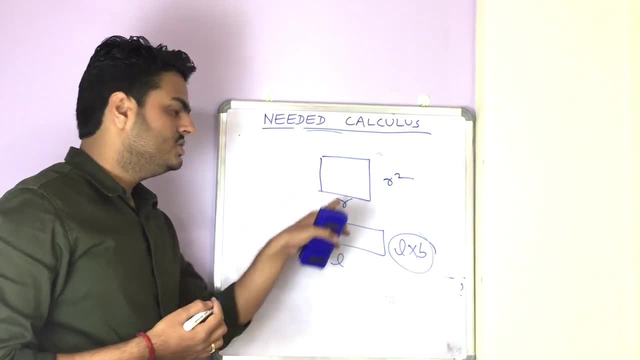 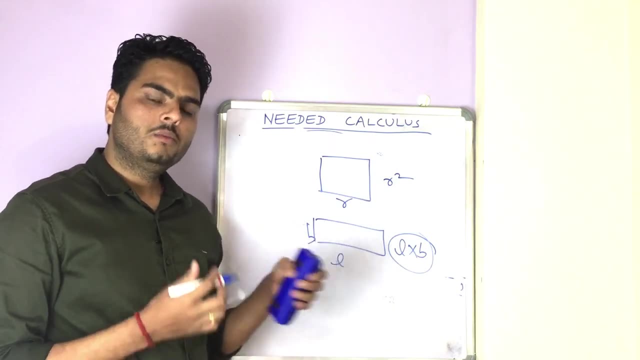 right, Because these are the defined shapes. hence there are defined formulas to calculate the area of these shapes. right? But in real world, in business scenarios, we do not always have some defined shapes. So we have to calculate the area of these shapes. right, But in real world, in business. 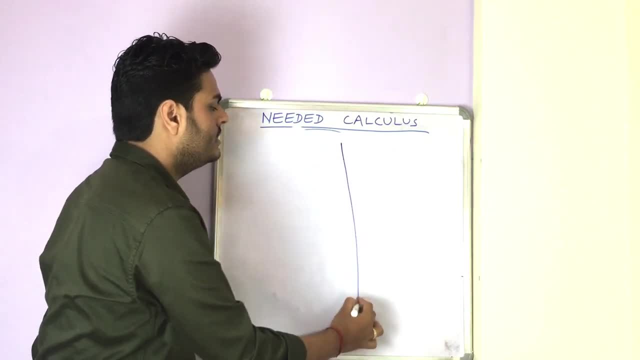 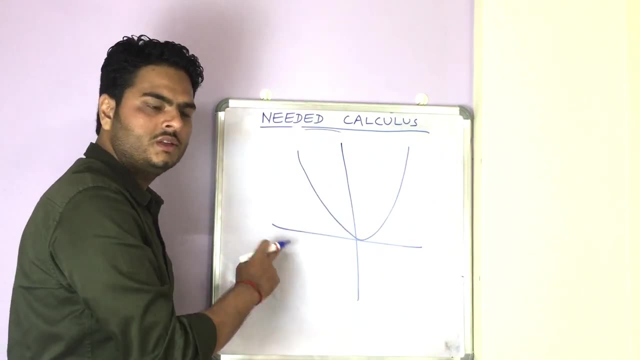 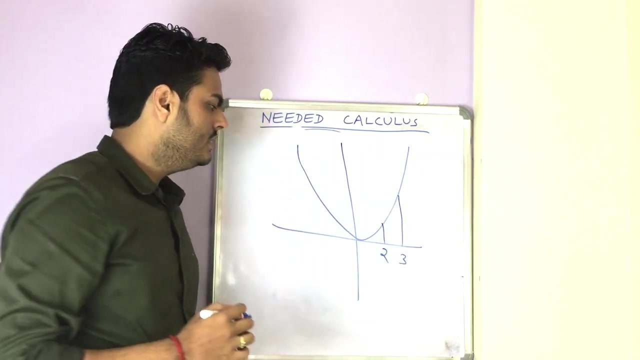 Let's go to our square function again and see how to calculate the area between two points. So this is the square function that we are talking about in this video and let's say: this is x is equal to 2 and this is x is equal to 3. Okay,